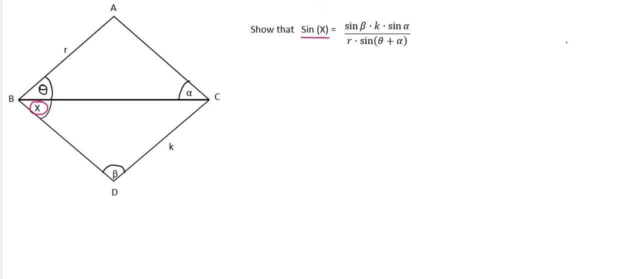 top triangle. So this is where you use your sin rule or cos rule, and remember that if they show you this angle- theta, for example, or alpha- that means that you can use that angle. Remember this whole section is about using letters instead of numbers. So that means you have those angles and 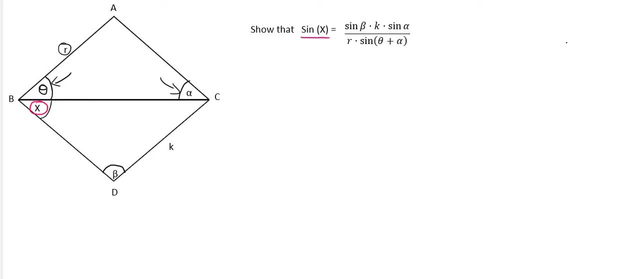 you also have this side over here. So remember we should always try use the sin rule first, as it's the easiest one to use between the sin and cos rule. So what we can do is we can see that side bc. well, that's opposite angle a, and then we have r, which is opposite. 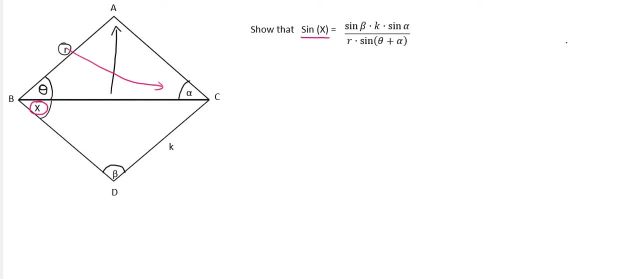 angle alpha. But now some students might say: but Kevin, we don't have angle a. Okay, you are right, at the moment we don't. but we do have angle b and we have angle c. So just using 180 minus those two, that'll give us angle a. So we can say that angle a is the opposite of angle b. So we can say that. 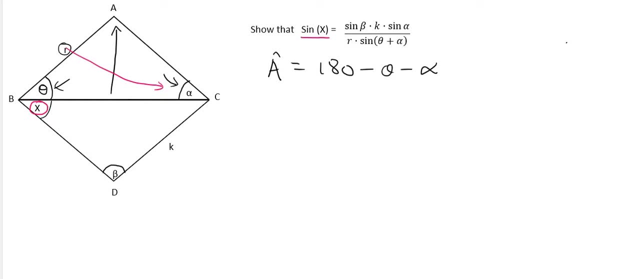 angle a is going to be equal to 180 minus theta minus alpha. Okay, that's just because of the sum of angles in a triangle. So now we can use the sin rule, So we can say that bc over the sin of its angle, which is the 180 minus theta minus alpha, is going to be equal to r over the sin of angle. 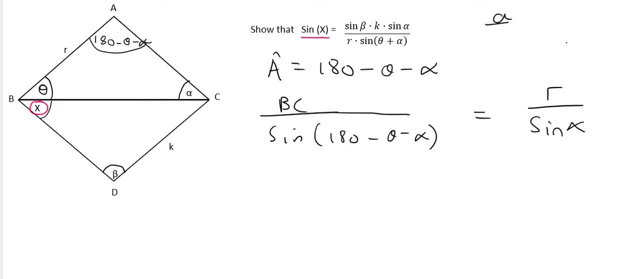 alpha. Okay, so you know where I'm getting that from. That's just using the normal sin rule: a over b over sin b. Okay, so that looks good. Now the goal of the question is to get- is to get bc by itself. So all I'm going to do is I'm going to take this part over here and I'm just going to. 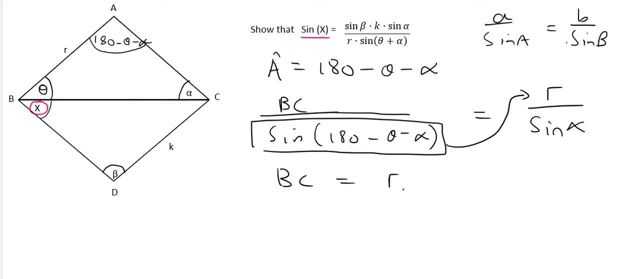 multiply it up to the top over there, And so bc is going to be equal to r times by the sin of 180 minus theta, minus alpha, And then all of that is going to be over sin alpha. What I want to quickly do now is just look at this section over here, This 180 minus theta, minus alpha, Because we can. 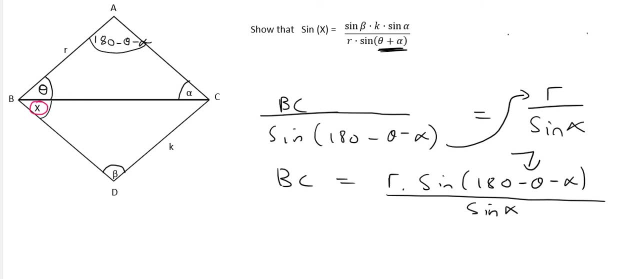 that's not part of the answer. They have it in a slightly different way, And many times they are going to do that in exams. Let me show you what they're doing there. So if we look at sin of 180 minus theta minus alpha, Now pay careful attention here, because once you understand this part, then 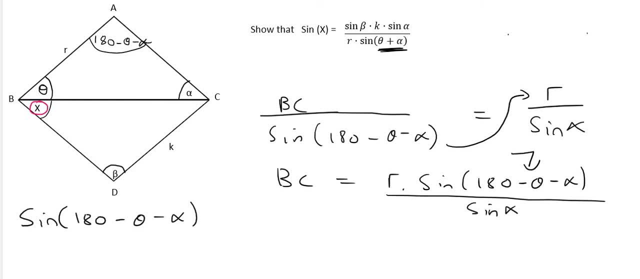 it's quite easy Because up till now, I'm sure this part has been a bit confusing. A lot of students get confused here, So what you want to do is take out a common factor within this bracket. So we're going to take out a common factor from that. 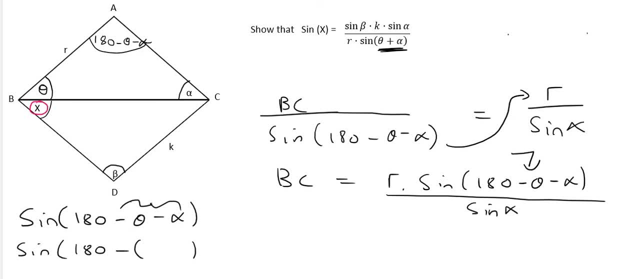 Section over there And what we're going to take out is a negative. We're then going to open up another bracket And what we'll be left with is theta plus alpha. Let me show you if that. let me. let's see if that makes sense. If we had to put the minus back into that bracket, that would give. 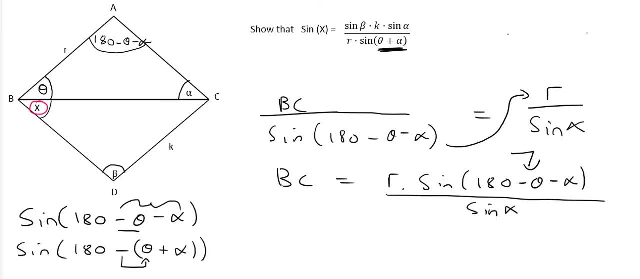 us minus alpha, I mean minus theta, which is what we had, And it would give us minus alpha, which is also what we had over here. So those two expressions, the top one and the bottom one, they are mathematically the same, They just look different. 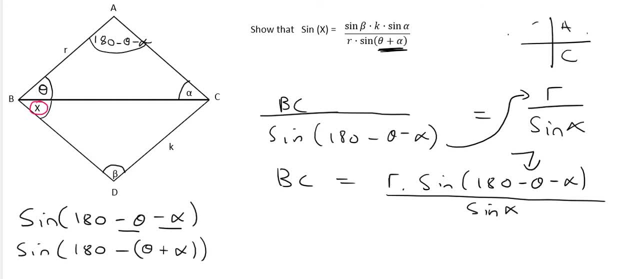 So let's take a look at that. So let's take a look at that. So we've got the sin of 180 minus x. If we had to reduce that, then that just becomes sin x. Okay, so that works for everything. So if we 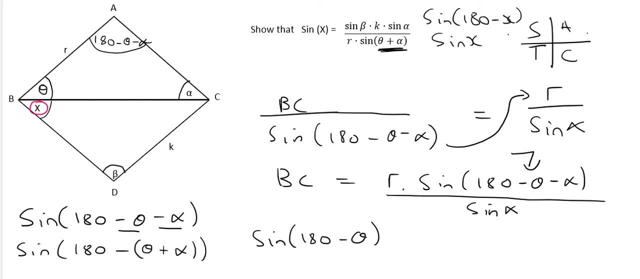 have a sin of 180 minus a smiley face, That's a smiley face- Then that just becomes the sin of the smiley face. If we have the sin of 180 minus z, then that just becomes the sin of of z. If we have the sin of 180 minus and then in brackets a plus b plus c, then that just becomes. 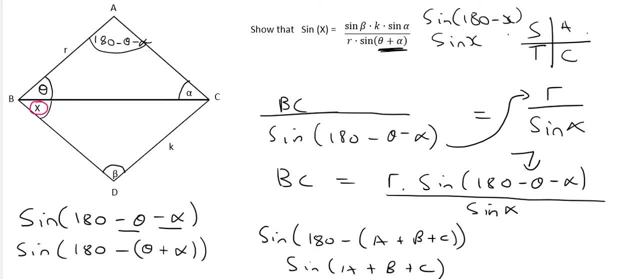 the sin of a plus b plus c. You see, so it becomes the sin of whatever's over here. So, with that being said, then this part here that I've got at the bottom left, well, that's just going to end up becoming sin of theta plus alpha. So we're going to transform this part over here into the sin of. 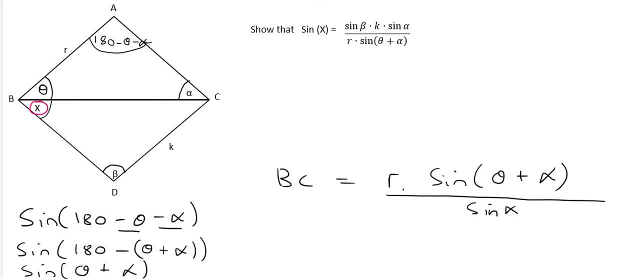 theta plus alpha, and there I've done that over there. Okay, so we've got bc. Now what we do is we work in the bottom triangle, but remember now we do have side bc. Our end goal is to find the sin of x, so we can try the sin rule again, because we've got k opposite sin x and then we've got beta opposite. 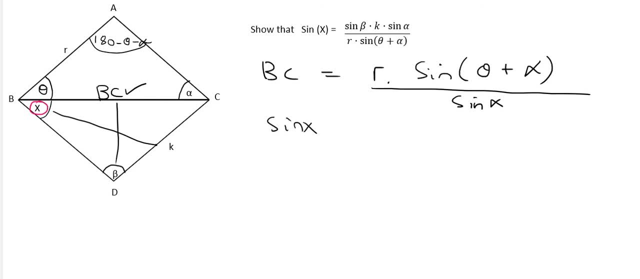 bc. So we could say that the sin of x over its opposite side, which is k, equals to the sin of beta over bc. Now I'll just call it bc. Now we're trying to get sin x by itself, so let's do that. The way I'll do that is: I'll multiply this. 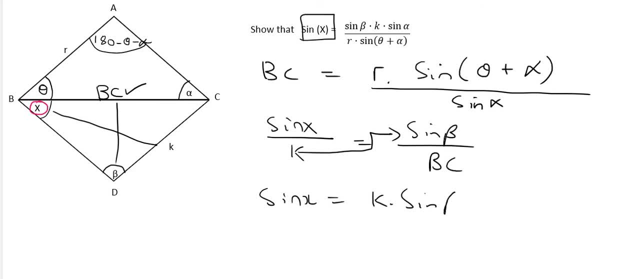 up to the top. So that's going to give you k sin beta over bc. Notice, I'm calling it bc for as long as I can because I don't want to have to write all this stuff down the whole time. Now, that okay, but 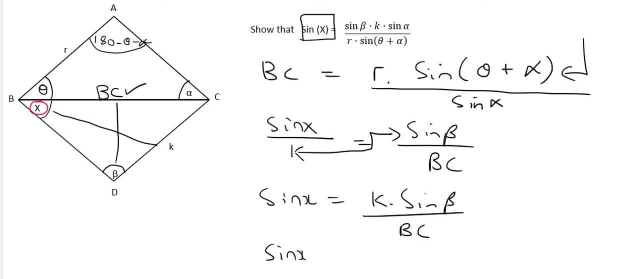 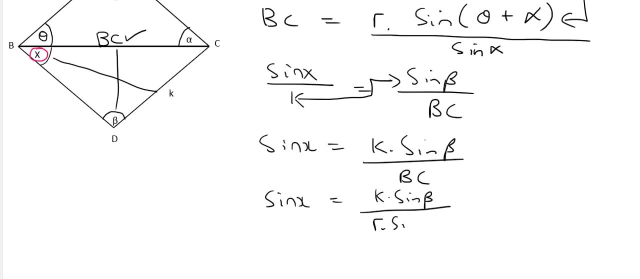 now we are at a position where we will have to fill in what bc is. So we've got k sin beta at the top, and then bc is going to be equal to r times by the sin of theta plus alpha, and then that's going to be over sin alpha, and then I'm just going to make 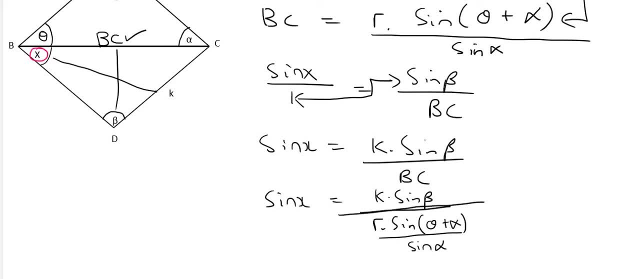 this line a little bit longer, because that's our main divide line. How do we now handle this now? So we've got a fraction on top of another fraction. Why do I say that the top part is a fraction? Well, I'm just going to write over here: We can think of k sin beta as k sin beta over 1, and then that's. 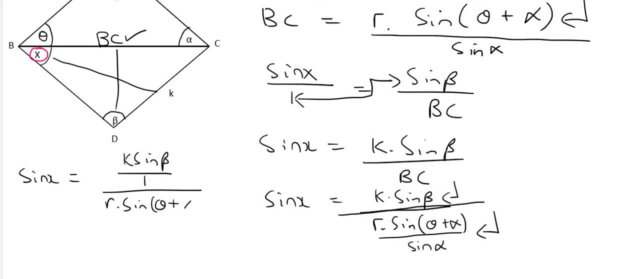 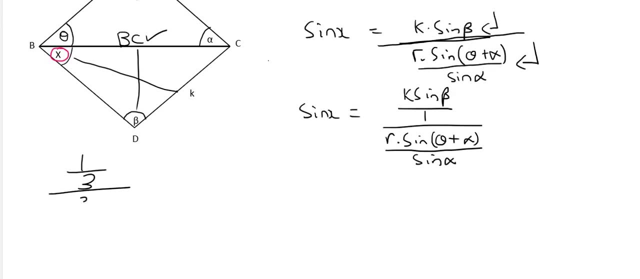 all over r times by the sin of theta plus alpha over sin alpha. Now remember, when you have a fraction on top of a fraction, then what you need to do is you do that little trick that we would have done many years ago in lower grades: You would leave the top part the same. so that's the. 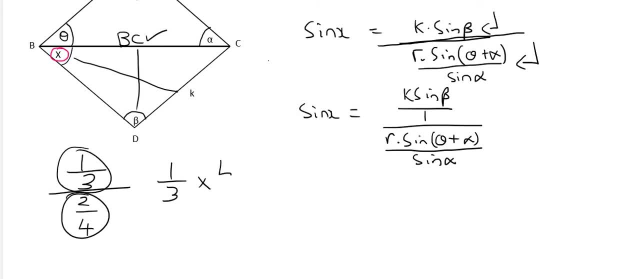 1 over 3.. Then you say times and you flip this part upside down to become 4 over 2.. So doing that over here we're going to end up with sin x equals to k times the sin of beta over 1.. 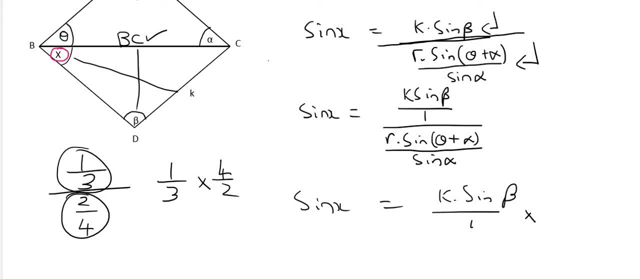 Times by the flipped over form of the bottom fraction. So that's going to be sin alpha over r times the sin of theta, or alpha plus theta, It doesn't matter. I've switched the order there, but that's okay. When you're plussing the order doesn't matter. and there we are pretty much at. 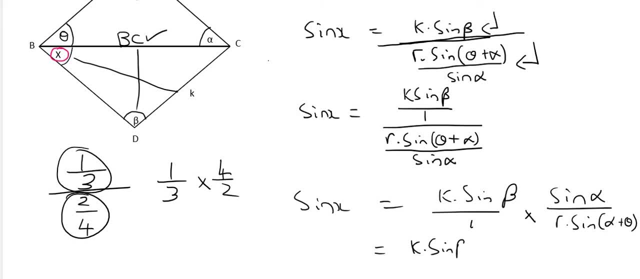 the answer. We can just multiply the top part together now. So that's just going to give us that over there, and then at the bottom we're simply left with r times by the sin of alpha plus theta.